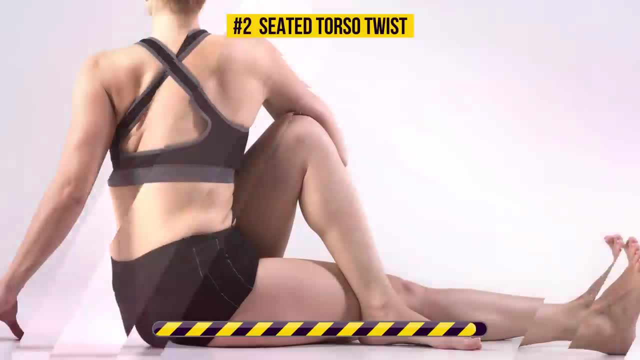 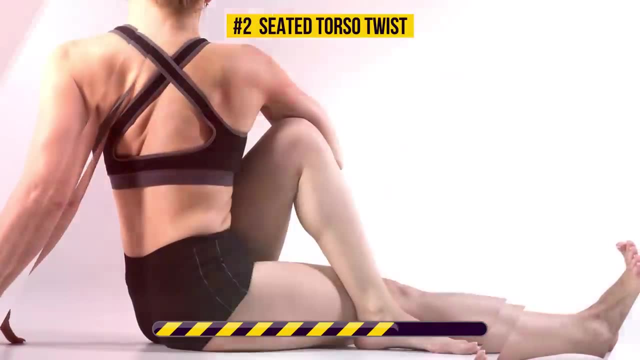 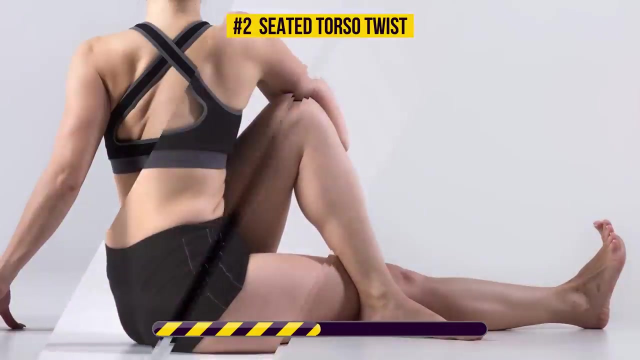 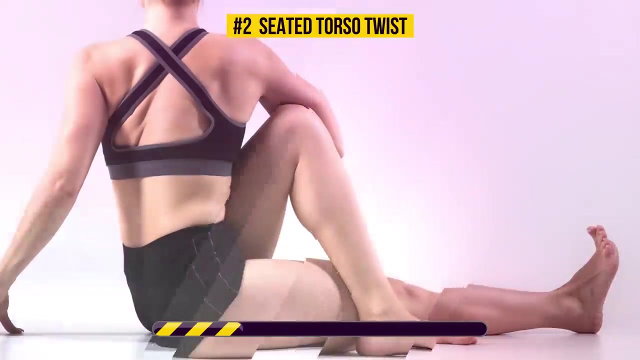 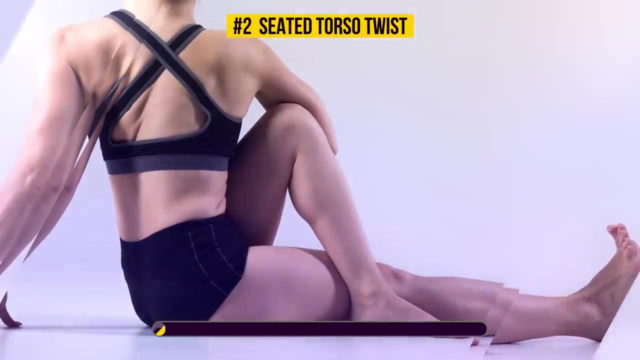 All clear, Then let's begin. This stretching exercise targets your back, abs and obliques. It engages all of your abdominal muscles and even reduces the risk of developing cardiovascular disease. We're almost done here And… perfect. Now let's move on to the next exercise. 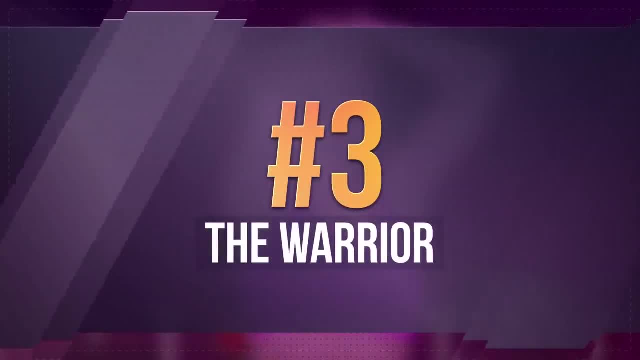 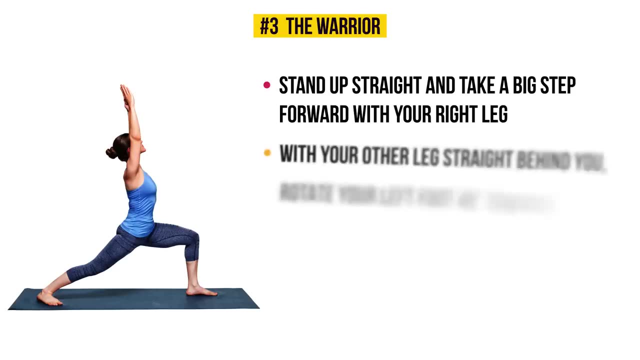 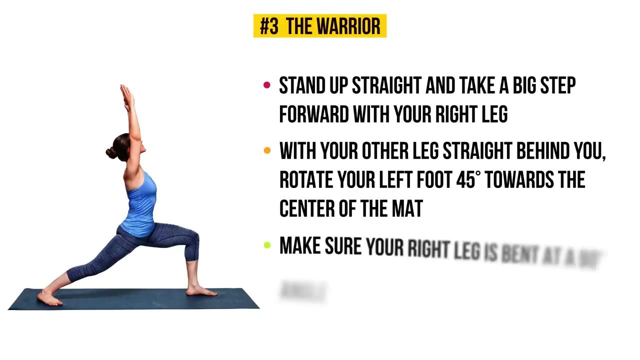 Exercise number 3. The Warrior Stand up straight and take a big step forward with your right leg, With your other leg straight behind you. rotate your left foot 45 degrees towards the center of the mat. Make sure your right leg is bent at a 90-degree angle. 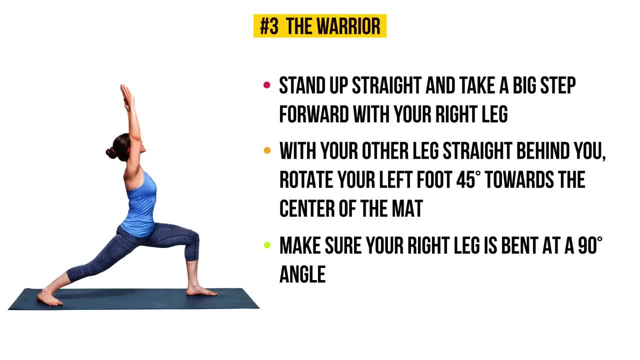 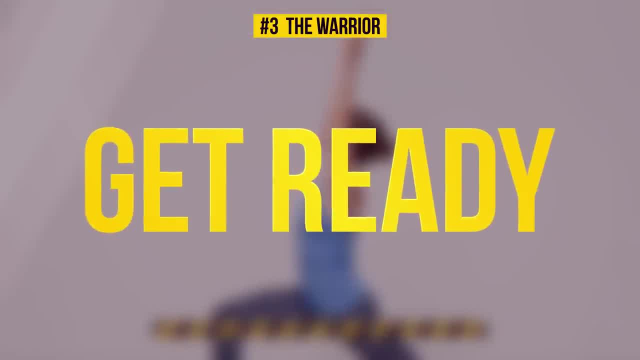 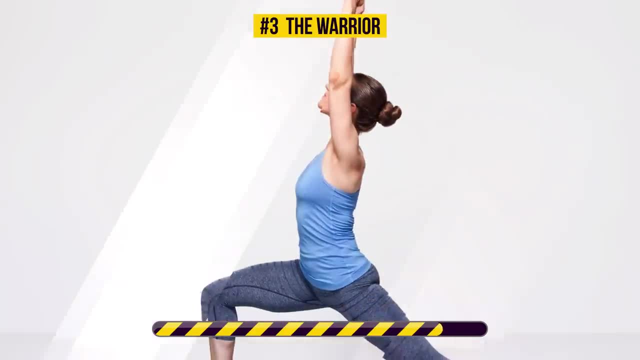 so that your knee is exactly above your ankle. From this position, reach your arms toward the ceiling and hold this pose for 30 seconds. All right, enough talking, Let's do it. This exercise works your hips, back and abs. 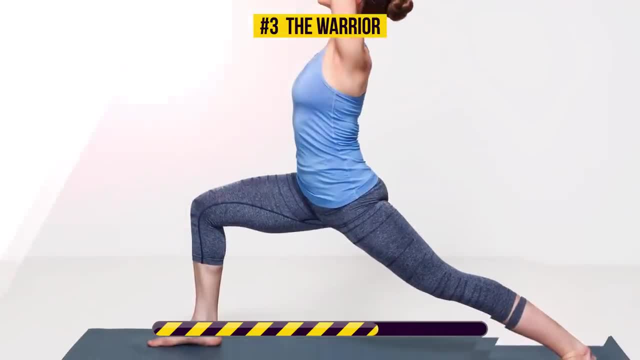 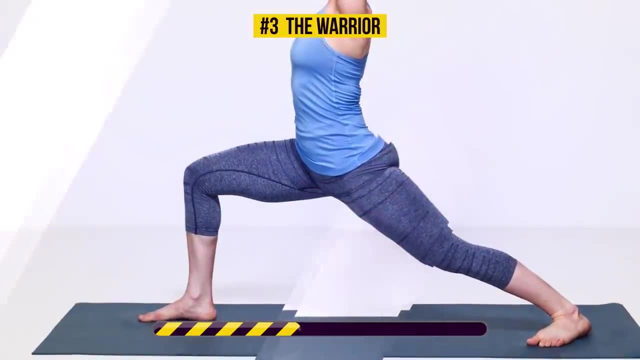 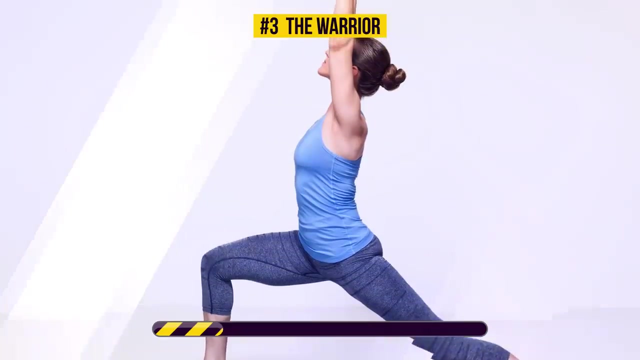 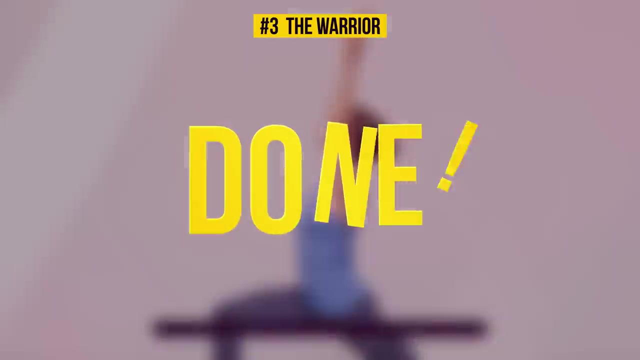 It also strengthens your core. The deeper the lunge you do, the harder your core works. The warrior pose improves your balance as well, And that's it. Take a deep breath And let's see what the next exercise is all about. 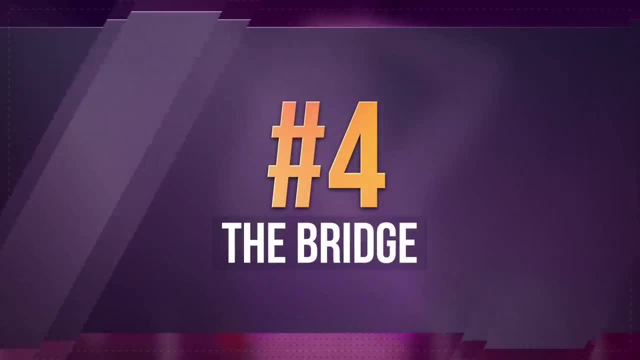 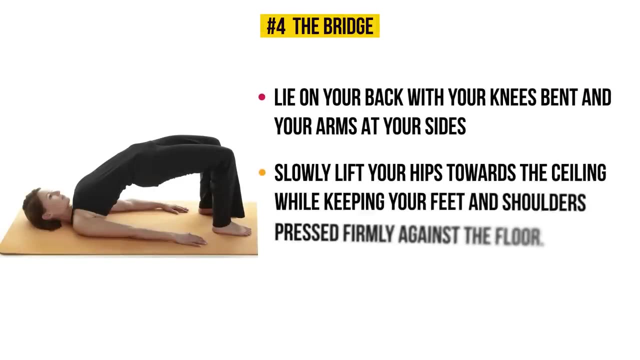 Exercise number 4. The Bridge. Lie on your back, with your knees bent and your arms at your sides. Lie on your back with your knees bent and your arms at your sides. Slowly lift your hips toward the ceiling, while keeping your feet and shoulders pressed firmly against the floor. 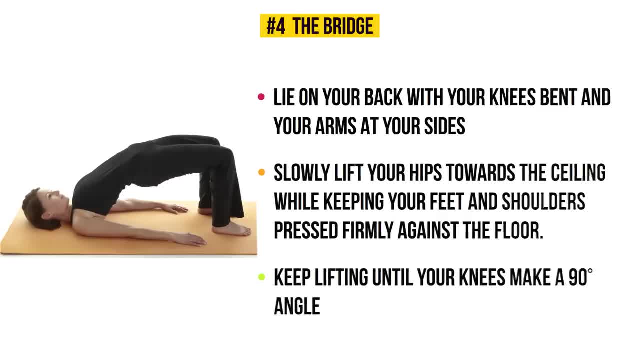 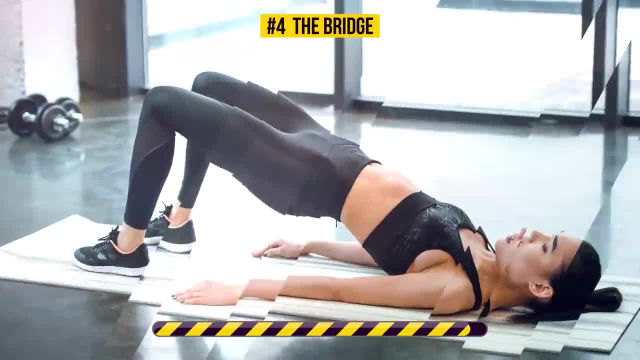 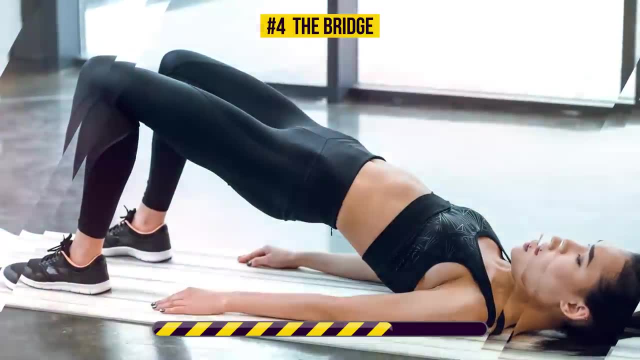 Keep lifting until your knees make a 90-degree angle. Think you can hold this pose for 30 seconds. Let's see. This exercise is a great workout for your glutes, legs and abs. It's especially known for toning and shaping the buttocks. 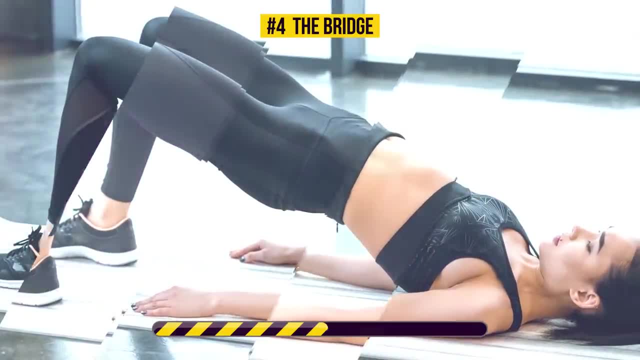 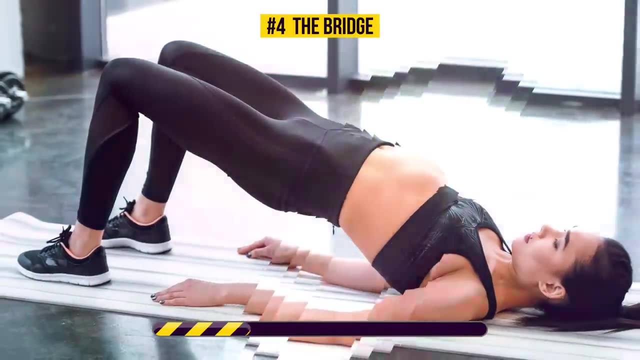 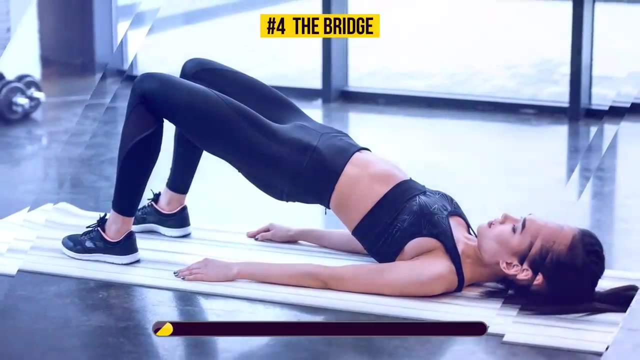 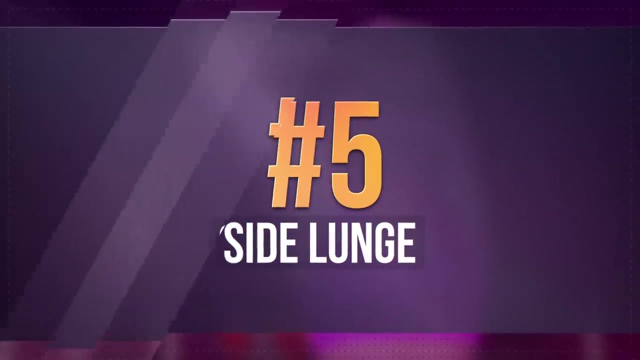 And no more back pain is a great bonus of this stretch too. And no more back pain is a great bonus of this stretch too. 3,, 2,, 1, and done Exercise number 5.. Side Lunge. 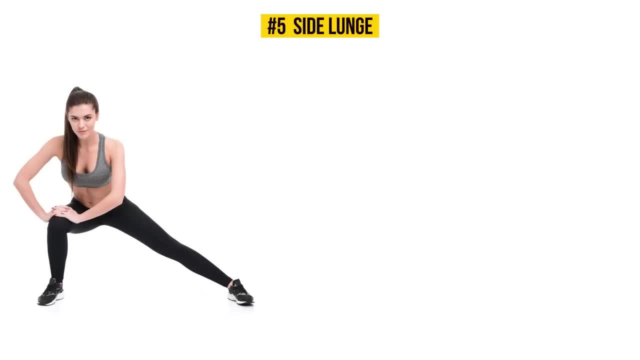 Exercise number 5. Side Lunge From a standing position. take a big step From a standing position. take a big step. Next, step to the right and dip your hips towards the floor until your knee is bent at a 90 degree angle. 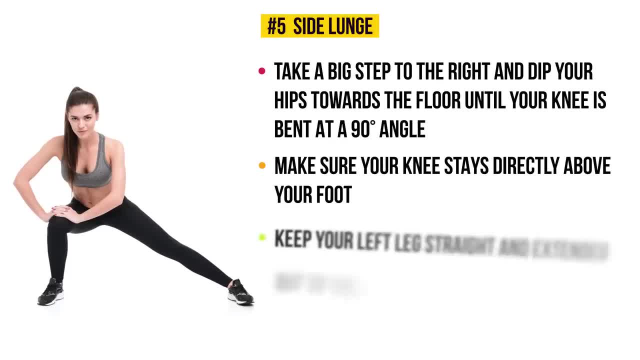 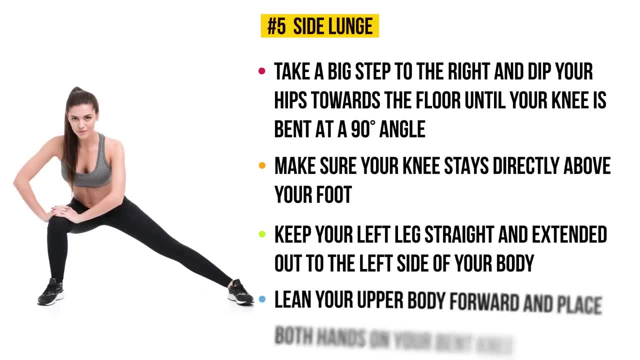 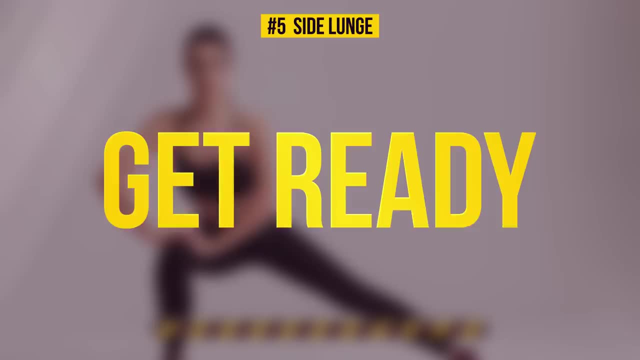 Make sure your knee stays directly above your foot. Keep your left leg straight and extend it out to the left side of your body, with your foot flat on the floor. Now lean your upper body forward and place both hands on your bent knee. Let's hold this pose for the next 30 seconds. 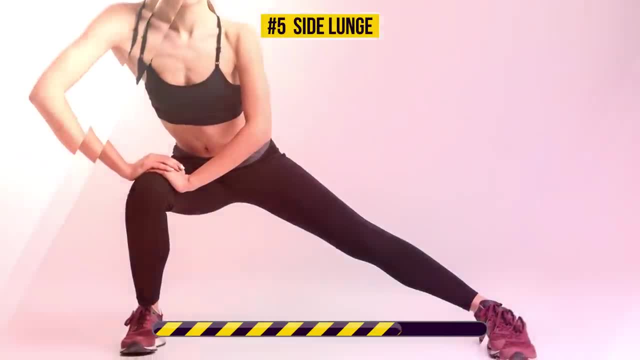 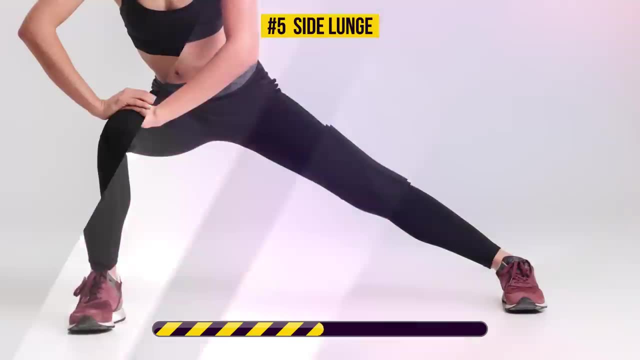 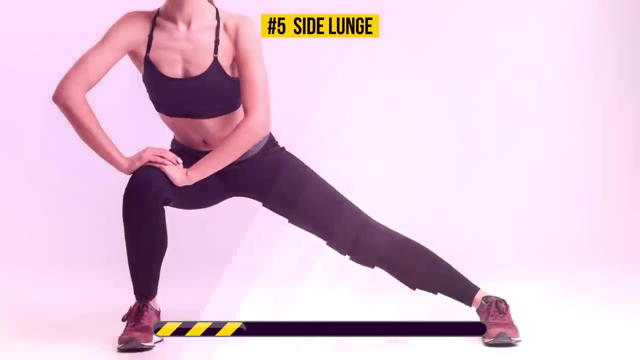 Side lunges have a positive effect on your hip flexors, quads and hamstrings. The main target, though, is your legs. This exercise will strengthen and tone them alright. Just 10 more seconds to go, Let's go. 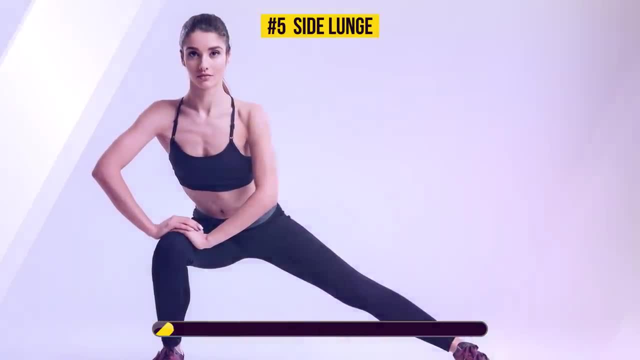 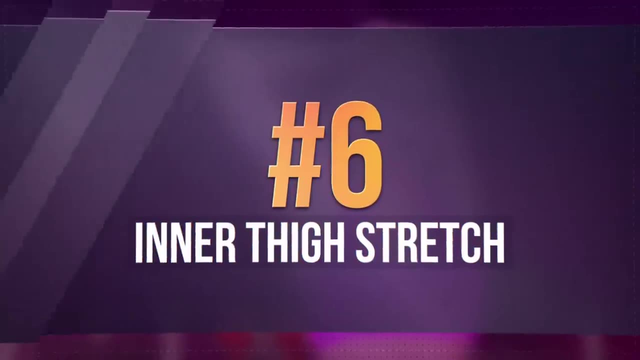 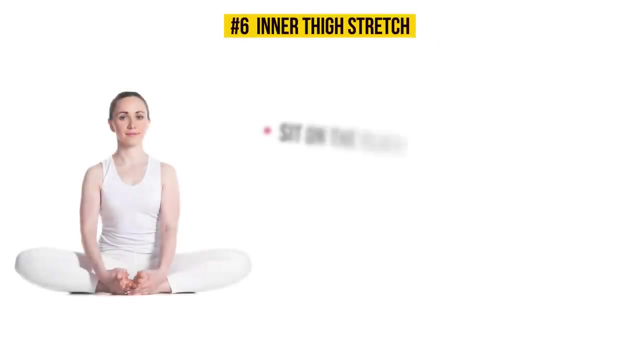 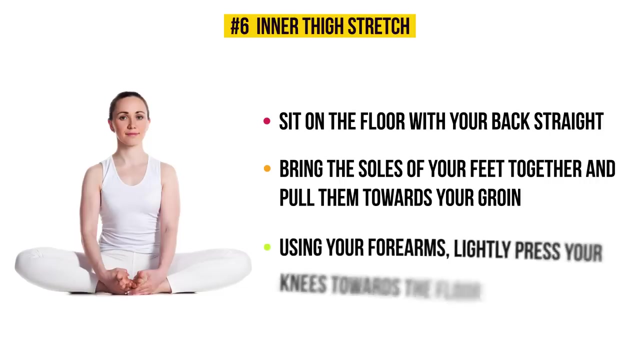 Good job. Exercise number 6. Inner thigh stretch. Sit on the floor with your back straight, Bring the soles of your feet together and pull them towards your groin, Using your forearms lightly press your knees towards the floor and you'll feel a gentle. 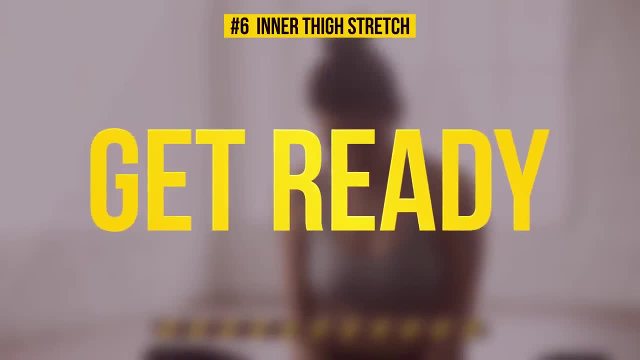 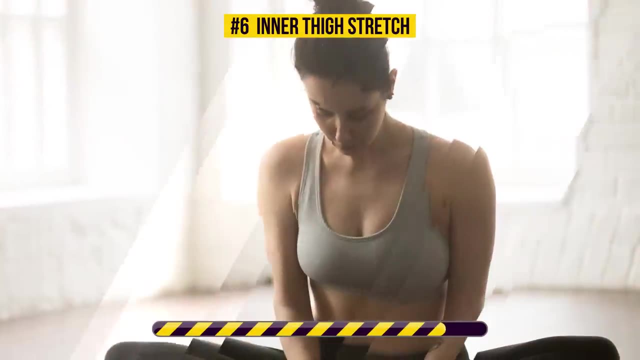 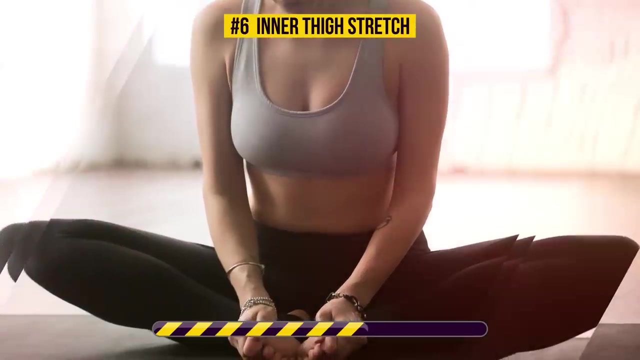 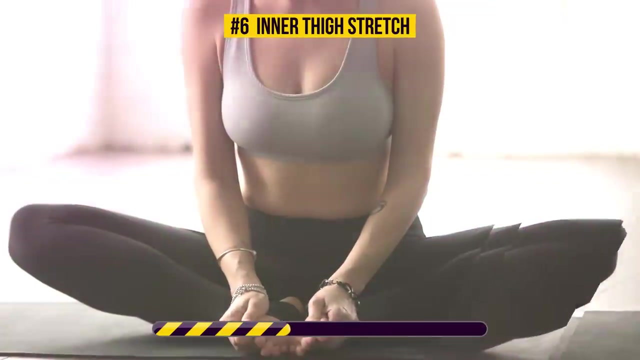 stretch. You know the drill: 30 seconds on the clock, Let's go. Stretching your inner and outer thighs is key for good flexibility. This pose in particular targets the muscles of your inner thighs and groin. If you aren't very flexible, doing this stretch regularly will change that significantly. 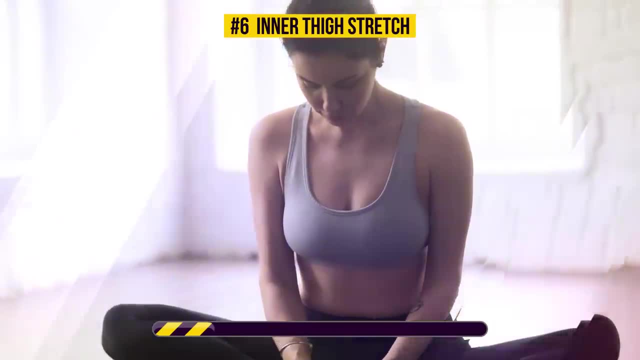 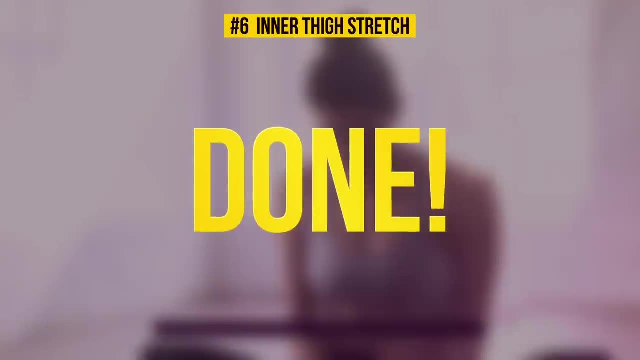 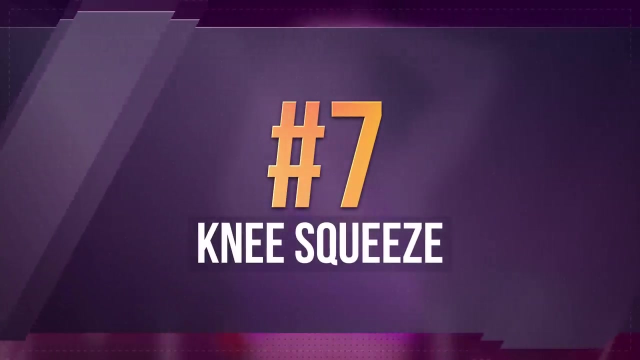 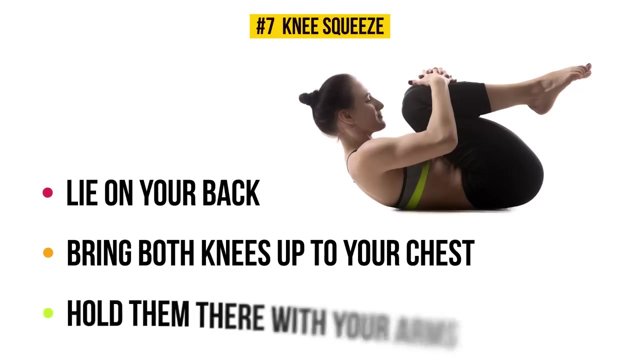 Just 5 more seconds. Well done, Exercise number 7.. Knee squeeze. Lie on your back, Bring both knees up to your chest and hold them there with your arms. You'll feel a little stretch, which, of course, is the whole point of our exercises. 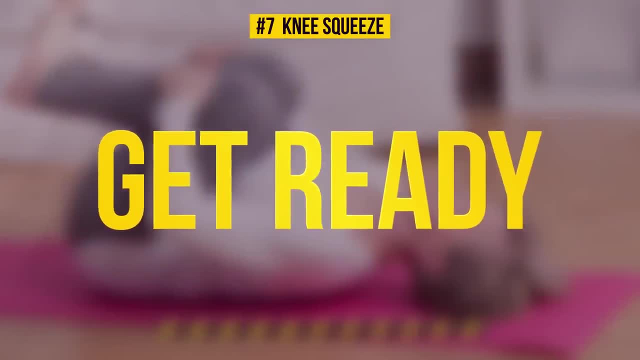 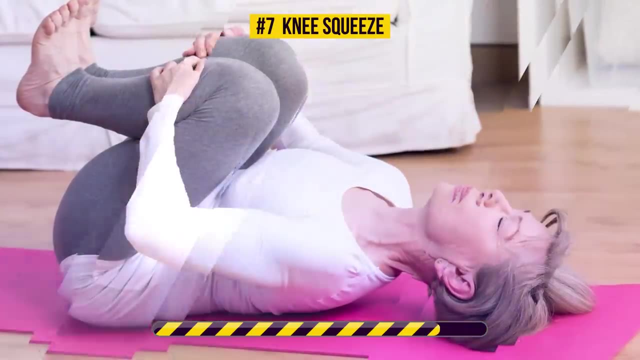 today. So let's squeeze our knees for 30 whole seconds. This exercise works your upper, middle and lower back muscles. You can do this with any of your muscles. You can do this with any of your muscles. It's also great at reducing and getting rid of knee pain. 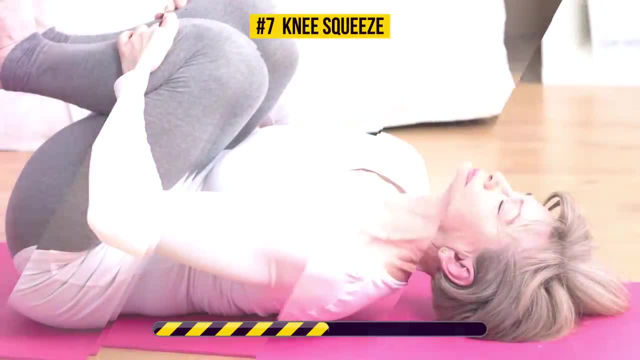 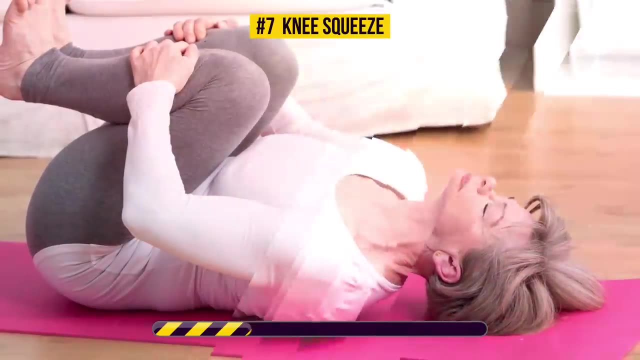 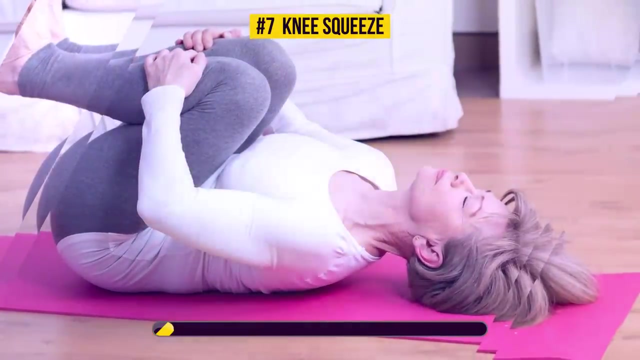 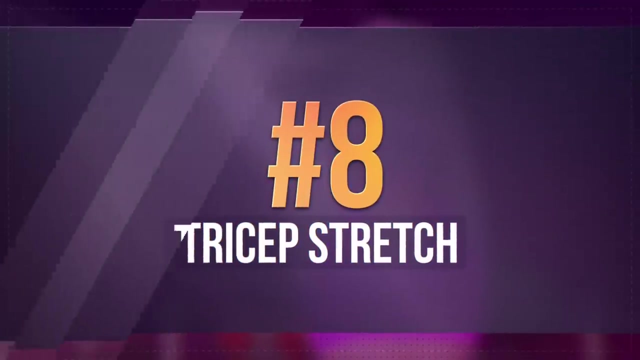 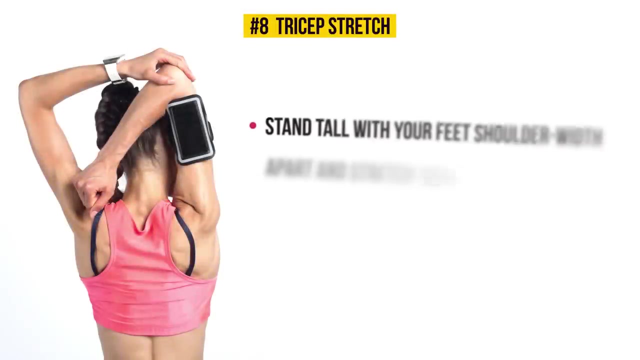 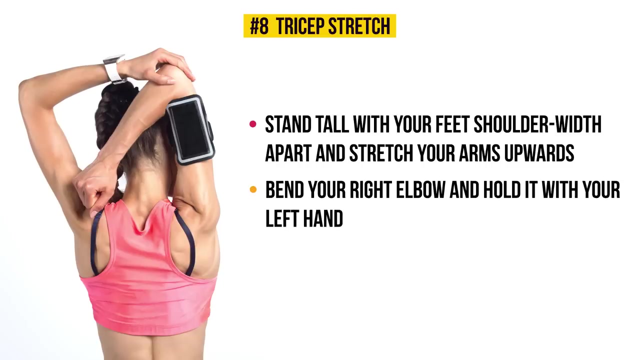 Just do it gently and know your limits. Hold it a bit more, and that's it Moving along. now, Exercise number 8. Triceps, Triceps, stretch. Stand tall with your feet shoulder-width apart and stretch your arms upward. Then bend your right elbow and hold it with your left hand. 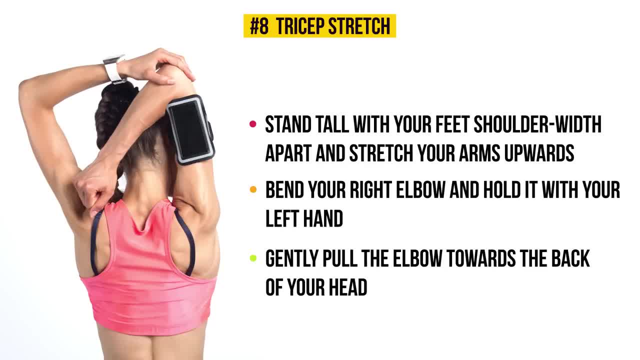 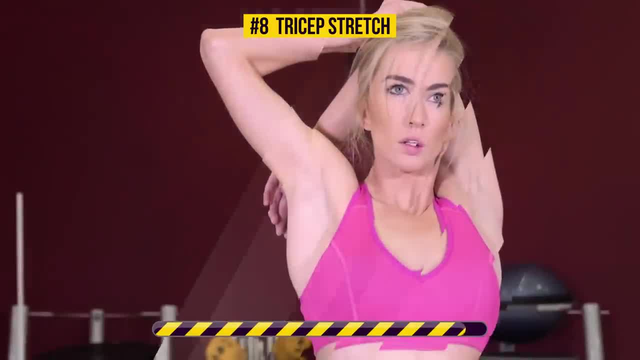 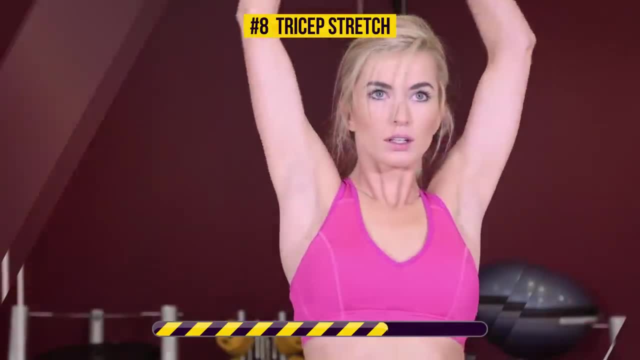 Gently pull the elbow toward the back of your head and hold this position for 30 seconds. 3,, 2,, 1, go. Tricep stretching targets your triceps As well as your back, shoulders and even your abs. 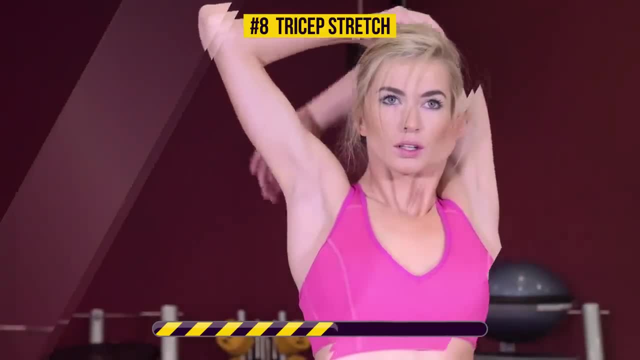 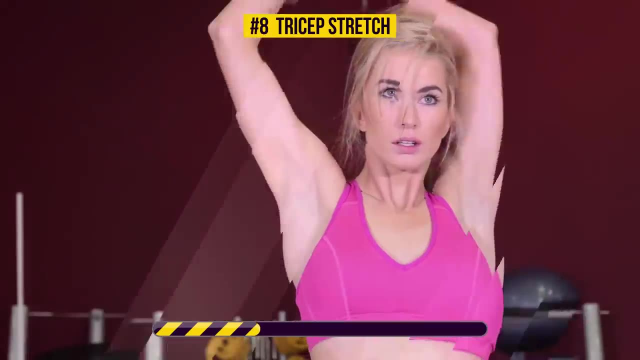 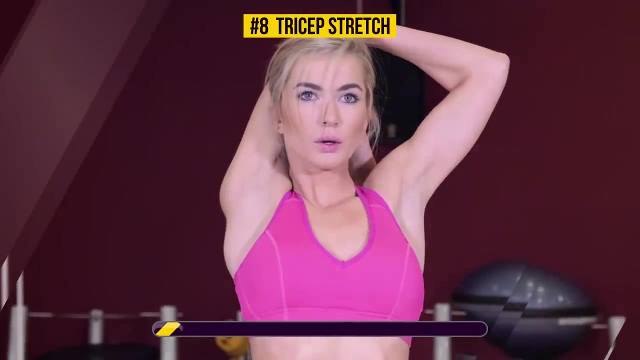 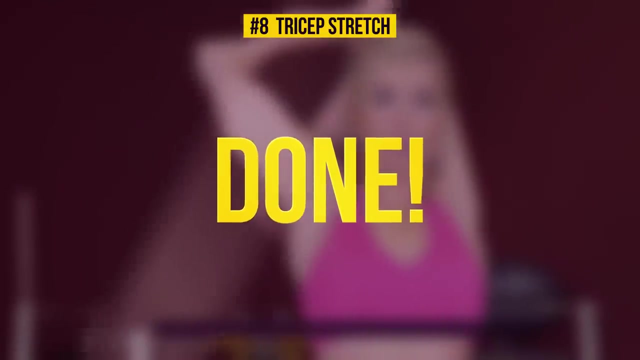 And that's it. Your back might be still a little heavy. This exercise improves flexibility and range of motion in your shoulders. Keep holding it just 10 more seconds And stop. Take a breather and then we'll move on to our next fat-burning exercise. 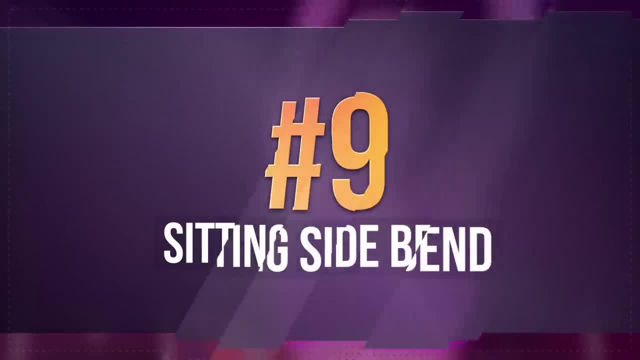 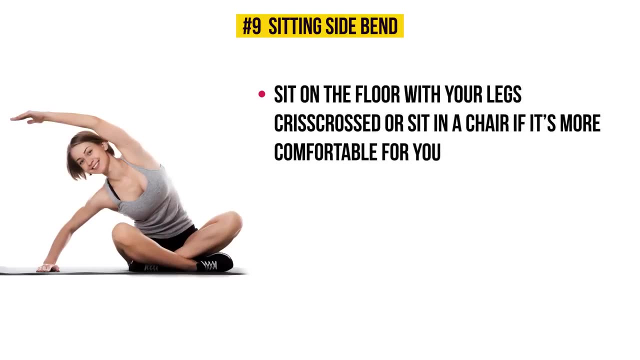 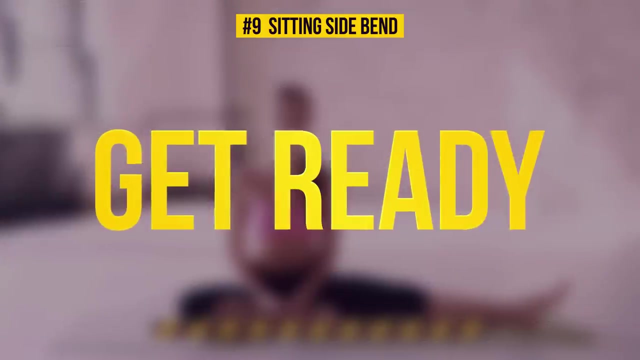 Sit on the floor with your legs criss-crossed, or sit in a chair, if that's more comfortable for you. Lift your left arm straight up above your head and bend to the right. A gentle stretch in your left side means that you're doing the exercise correctly. 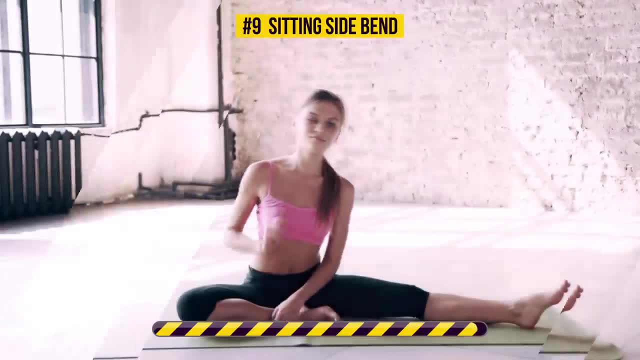 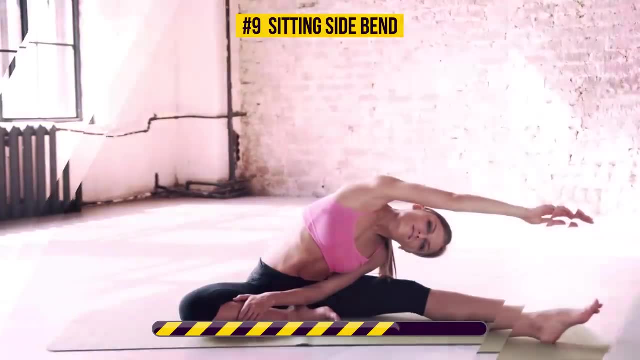 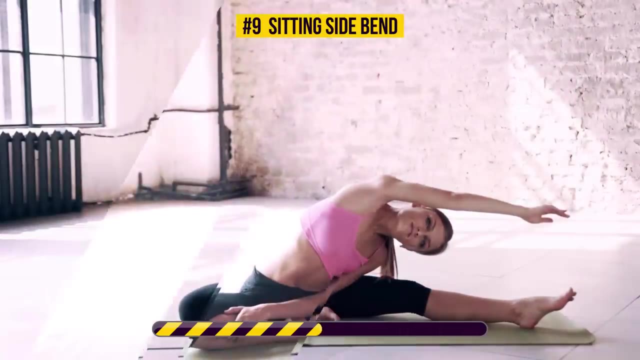 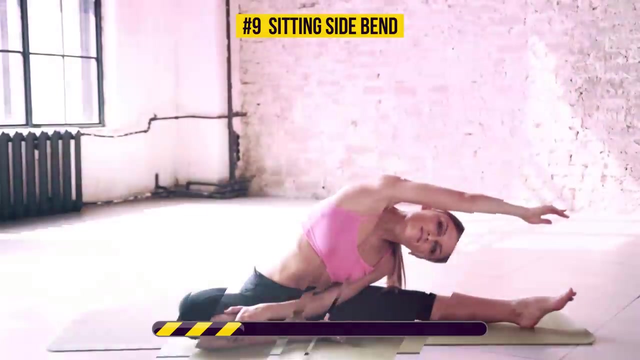 Half a minute on the clock starts now. Sitting side-bend gives a good workout to your obliques, back, shoulders and abs. It also helps relax your mind and relieve any stress or anxiety. Keep going, you're doing great. 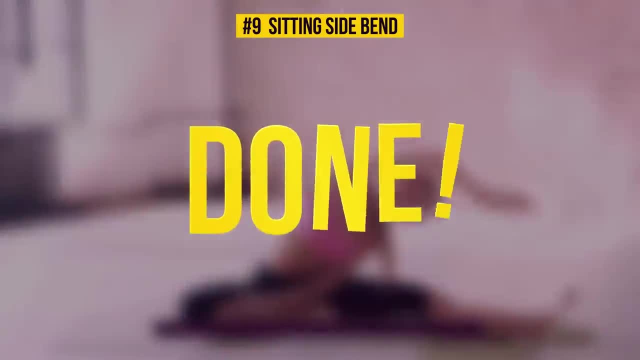 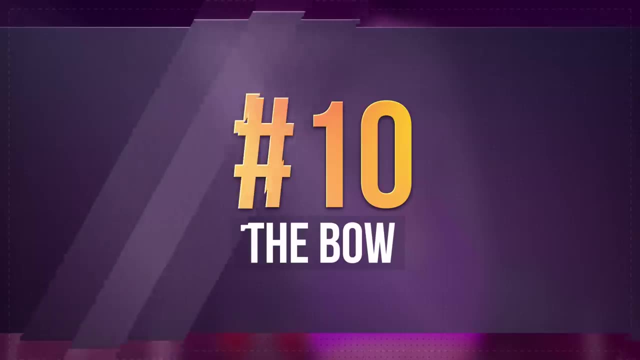 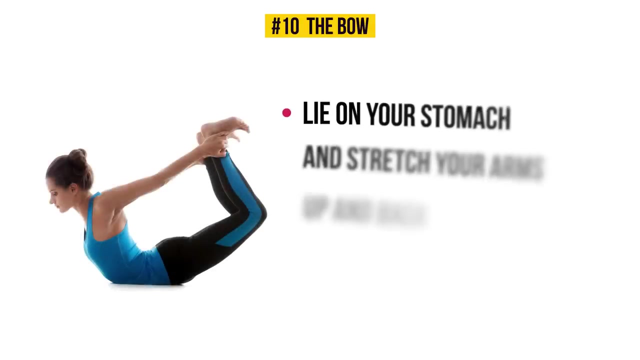 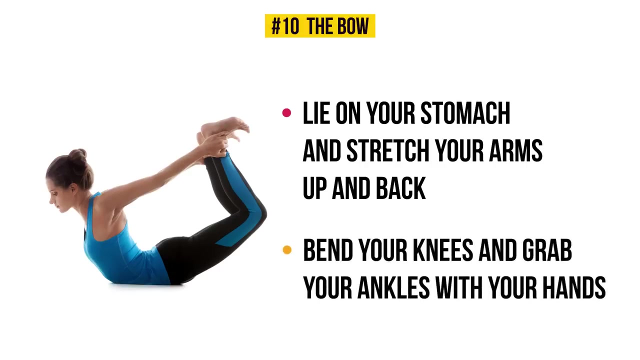 And that's it. Hang in there. we only have 3 more exercises to go. Exercise number 10, the bow. Lie on your stomach and stretch your arms up and back, Bend your knees and grab your ankles with your hands. Just like with all our previous exercises, we're going to hold this pose for 30 seconds. 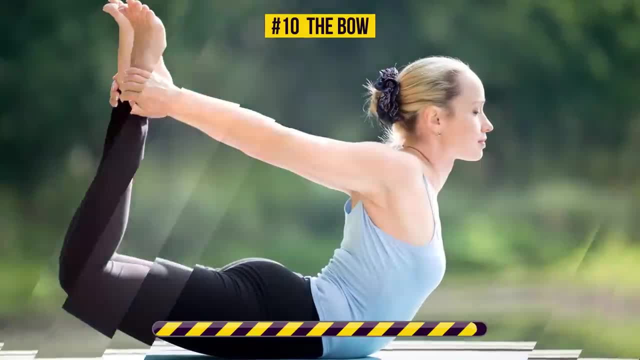 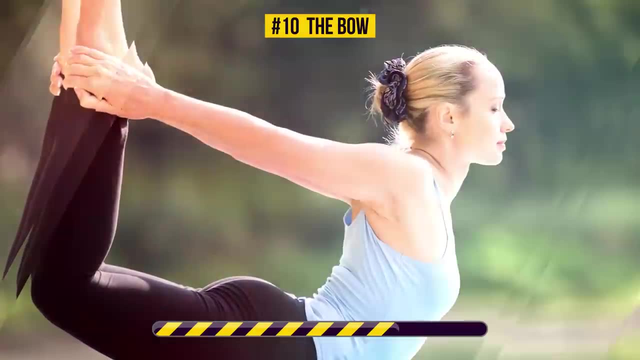 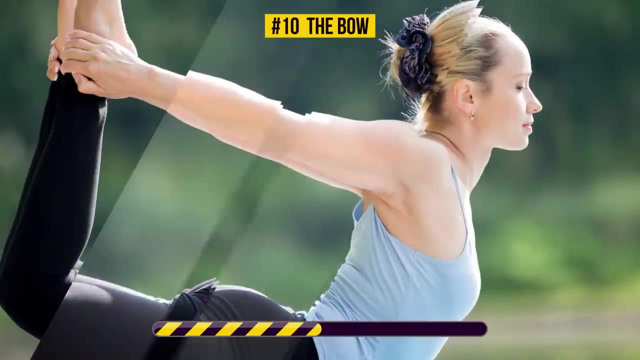 Are you ready And go? The bow pose targets your abs, back and hips. While you're doing it, don't forget to keep the tops of your shoulders away from your ears. If you do the exercise regularly, it'll improve your posture and tone your abs. 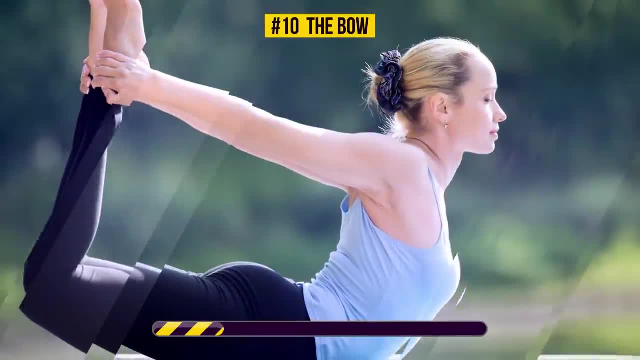 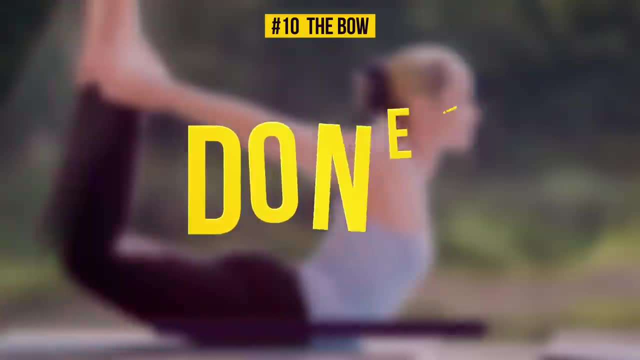 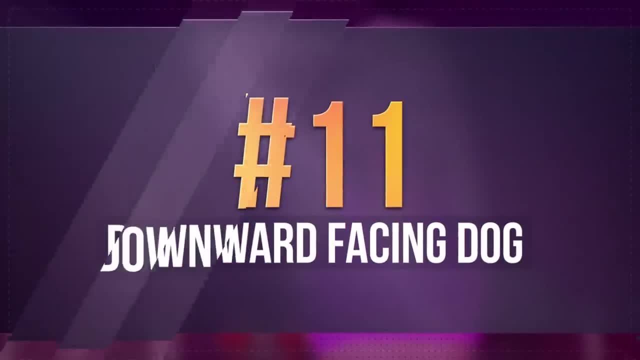 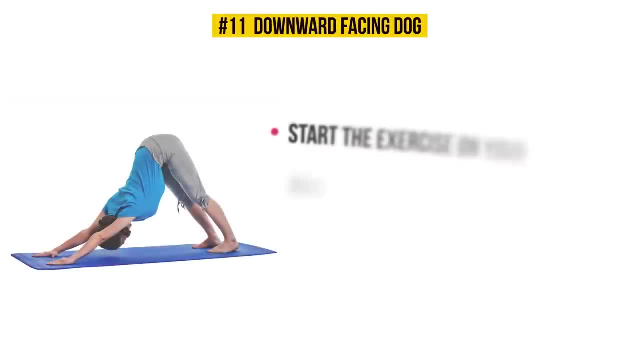 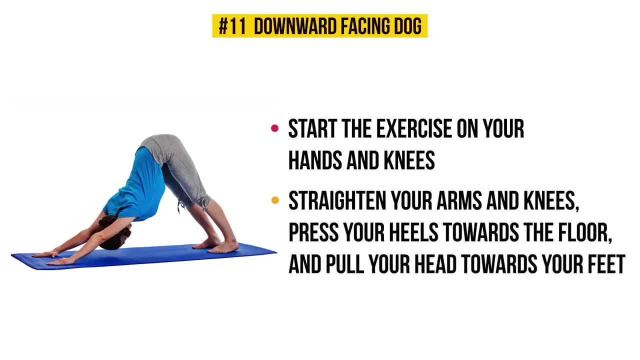 Exercise number 11, downward-facing dog. Start the exercise on your hands and knees. As you exhale, straighten your arms and knees, press your heels toward the floor and pull your head toward your feet. How many seconds are we going to hold this position? 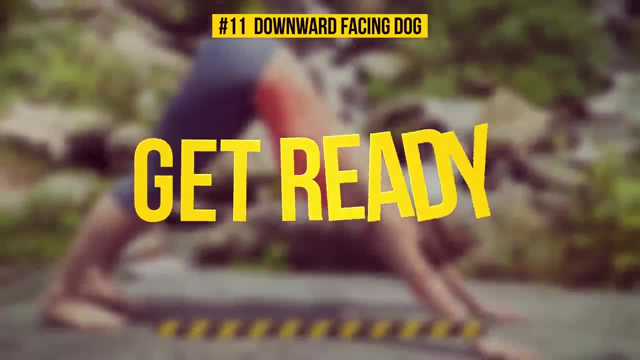 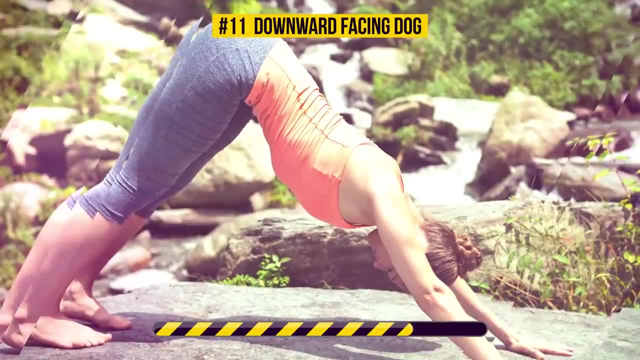 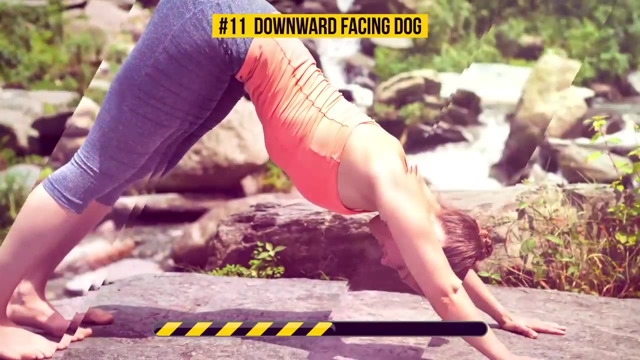 You don't know. You don't know You got it. 30, off you go. This pose targets your legs, hips, back, shoulders and arms. It improves digestion too. Besides the physical stuff, it also has a great effect on your emotional state, helping. 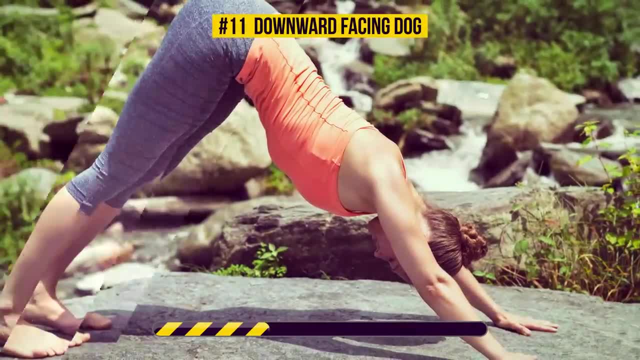 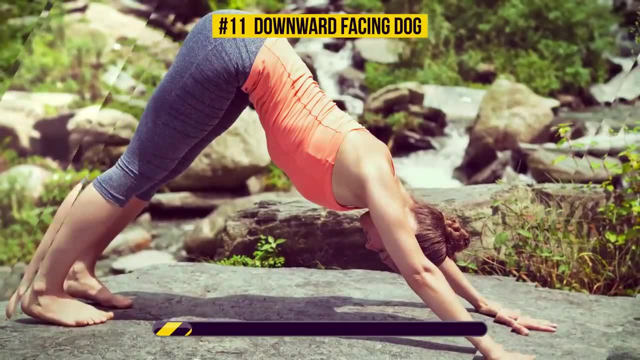 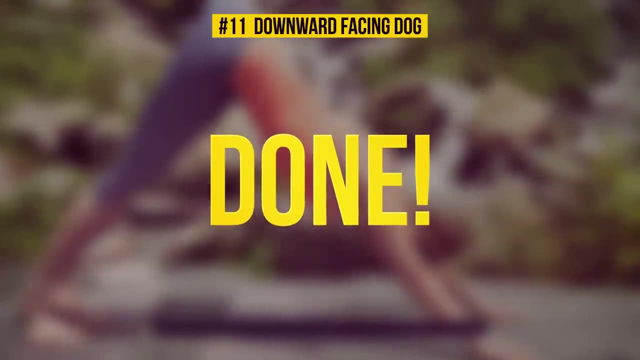 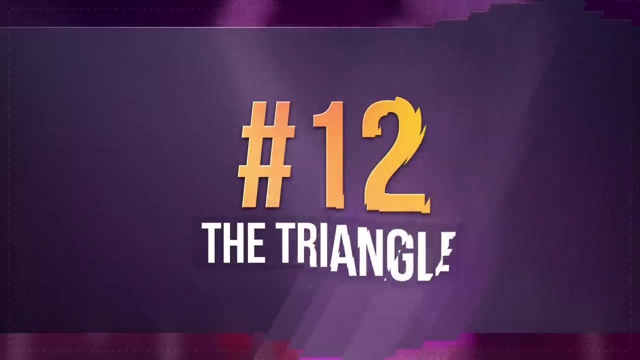 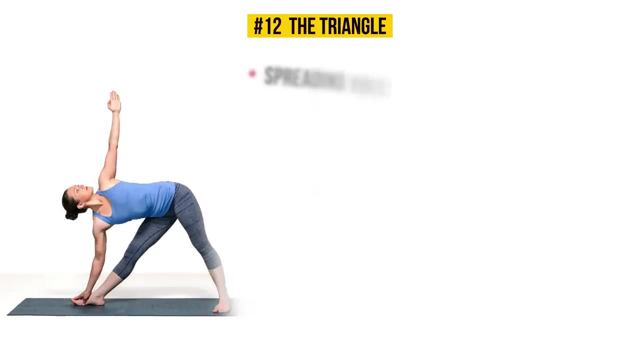 you deal with depression and stress, Don't forget about your breathing And time's up Props to you for coming this far with us. Let's conclude this workout with our final exercise, Exercise number 12, the triangle. Start by standing on your mat and spreading your feet really wide. 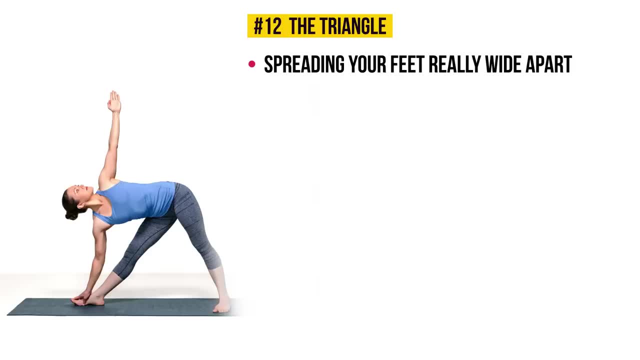 There should be about a 4-foot distance between them. Turn your left foot outwards 45 degrees and your right foot 90 degrees. Hold your arms parallel to the floor, breathe in and start stretching to the left as if you're trying to reach something. 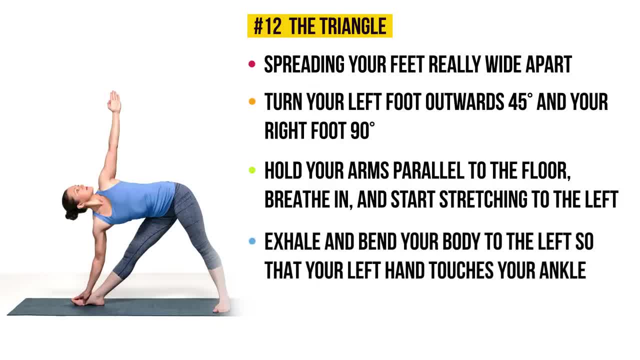 Then exhale and bend your body to the left so that your left hand touches your ankle or a yoga block, if that's more comfortable. After that, stretch your right arm towards the sky. Keep looking up and hold this pose. Stay in this position for the next 30 seconds. 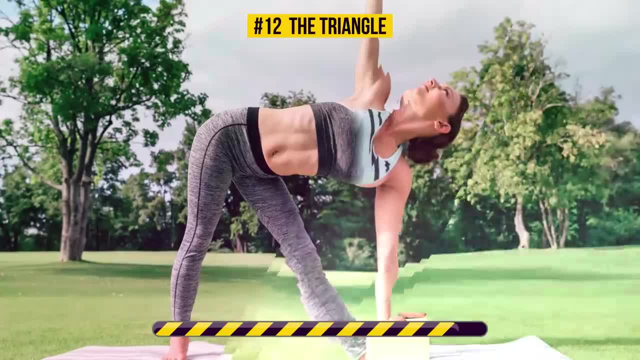 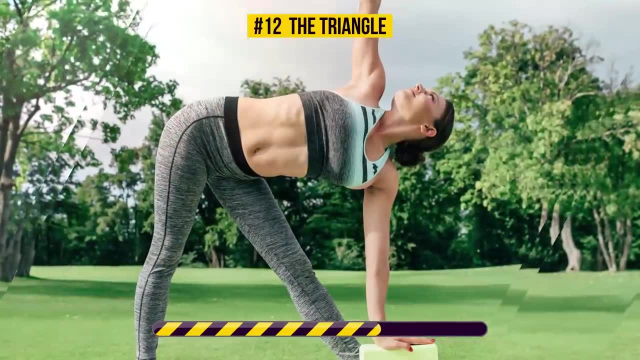 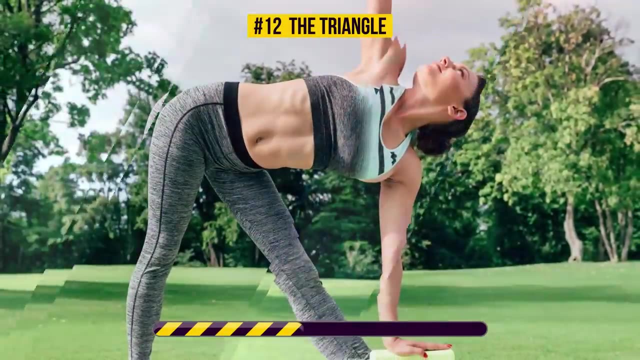 Time's ticking. This exercise works your legs obliques, hips, shoulders and chest. It also gives your sides a good deep stretch And, like most yoga poses, it helps relax your brain and calm your emotions. Let's do it. 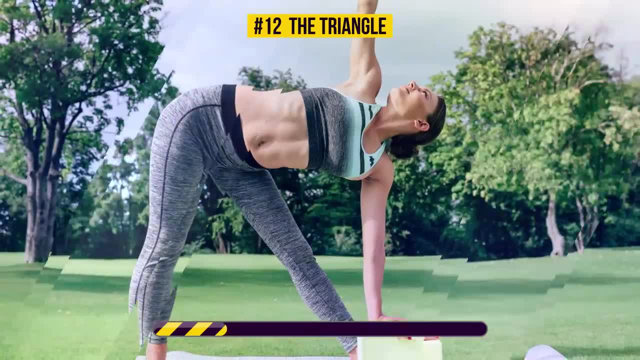 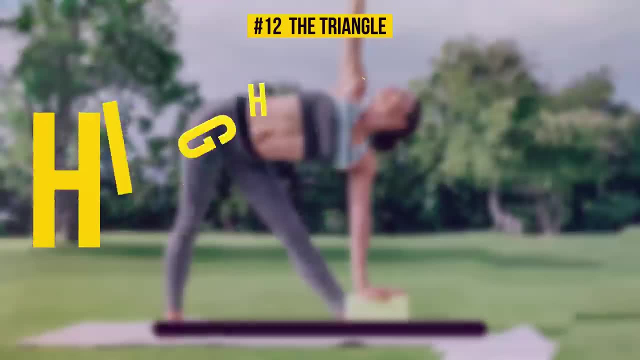 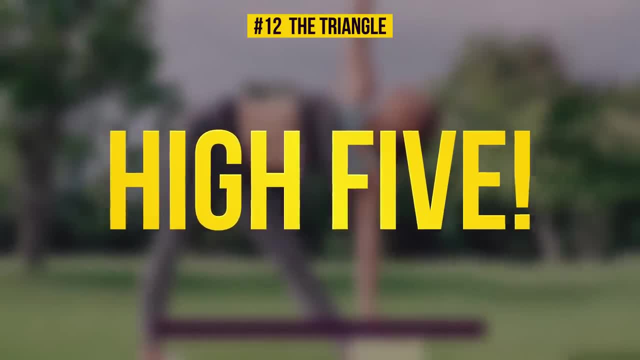 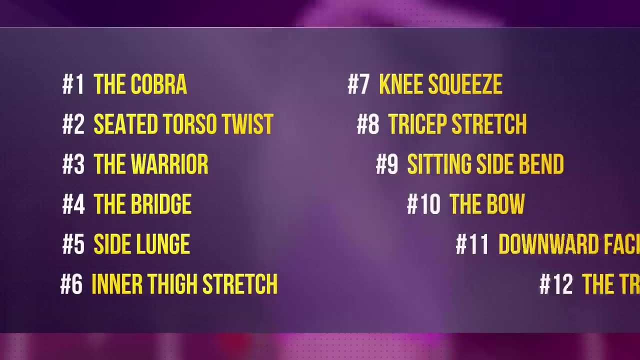 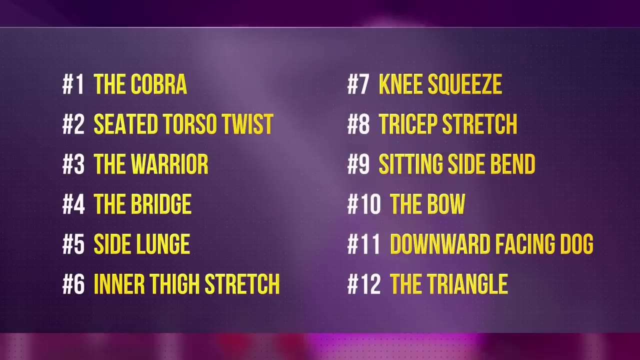 So that was the last exercise for today's workout. High-five for being awesome and sticking through it. Don't forget to come back to this video at least once a week and do these exercises with us. They have Tons of health benefits that will allow you to achieve your dream body within. 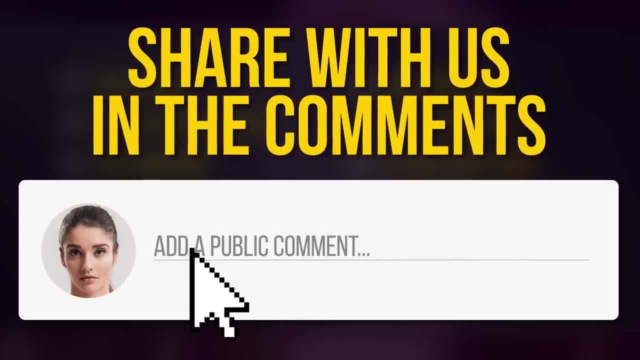 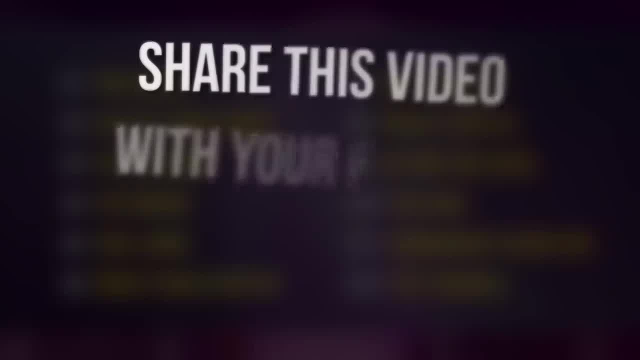 weeks fit. Tell us in the comment section below. Don't forget to share this video with your friends. You can even do this simple workout together. Remember to always stay on the Bright Side of life and we'll see you soon.